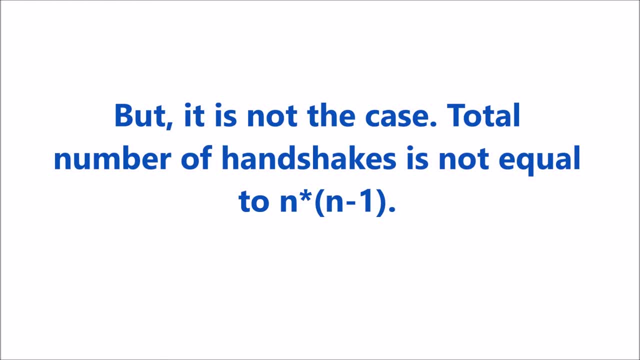 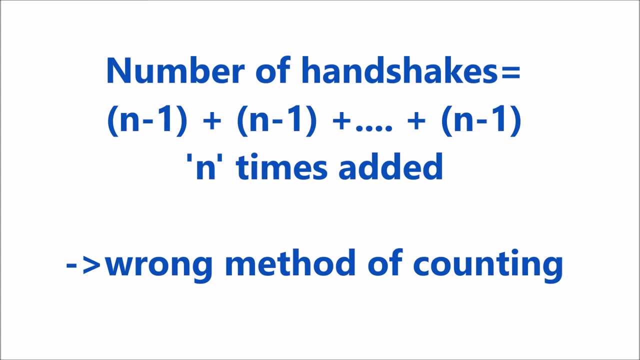 But it is not the case. The total number of handshakes is not n into n minus 1.. Why so? Because when we count the total number of handshakes in that manner, we can see that every handshake is counted twice. 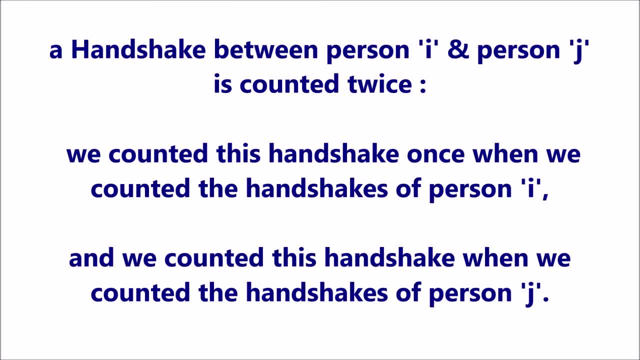 For example, a handshake between a person i and a person j is one handshake right And we counted this handshake twice in our method, because we counted this handshake when we counted the number of handshakes for the person i, And also we counted this handshake when we counted the number of handshakes for the person j right. 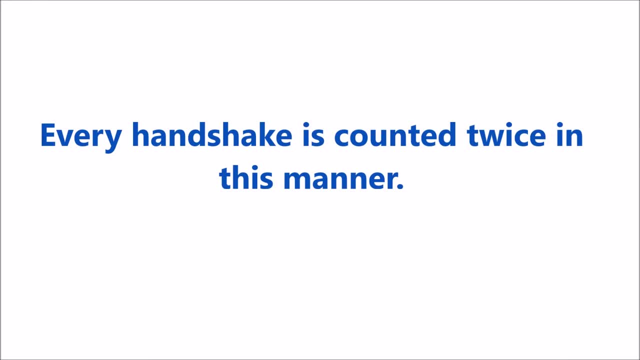 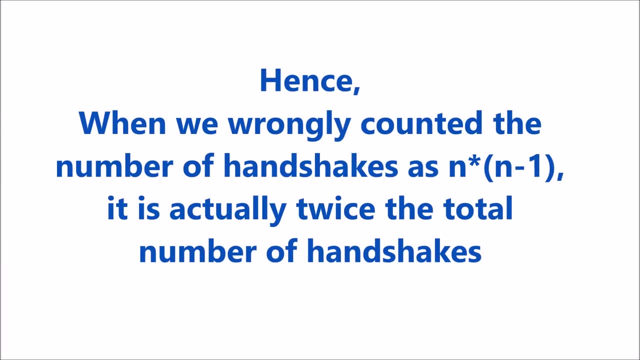 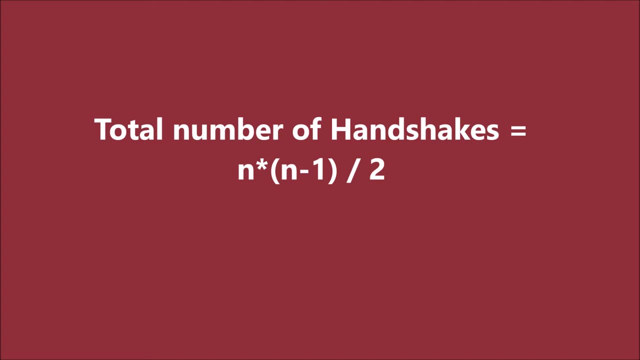 That's why every handshake is counted twice in this manner. For example, when we counted the number of handshakes as n into n minus 1, it is actually twice the original number of handshakes. That means 2 into number of handshakes is n into n minus 1, and the number of handshakes is n into n minus 1 by 2.. 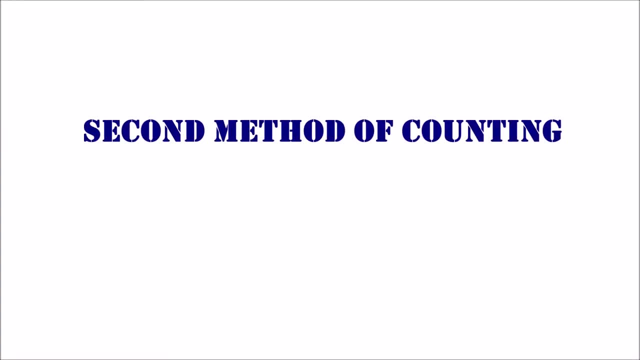 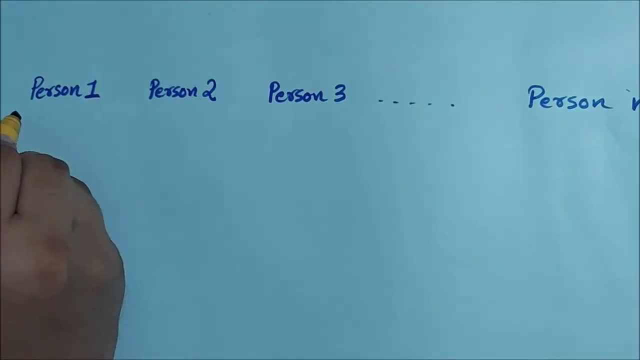 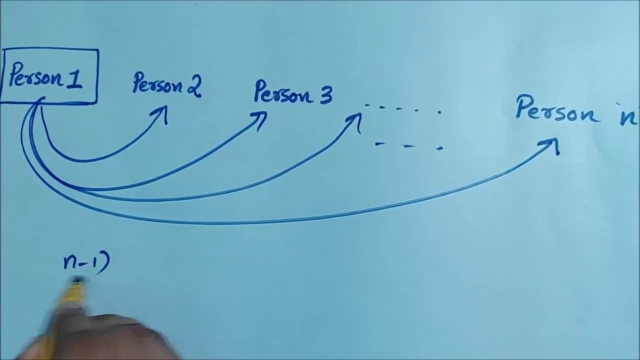 Now we will see a second way to count the number of handshakes. Let's visualize n persons standing in a row- okay, And the first person will go to every other person and makes the handshakes Okay. So n minus 1 handshakes we have to count on the behalf of person 1's handshake right. 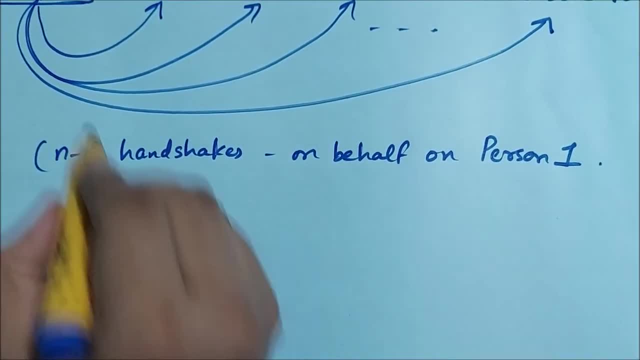 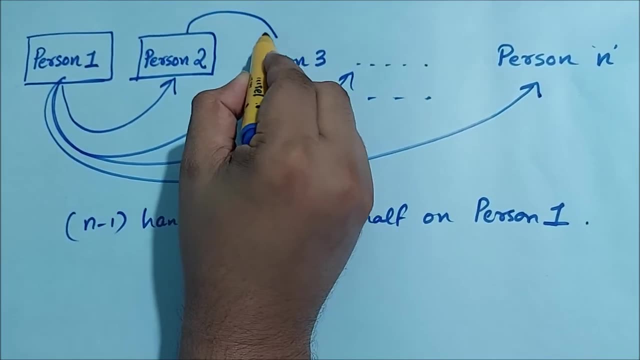 Okay, Now next person 2's turn. Person 2 will not make handshake with person 1 again, because that handshake has already been done. right Now, person 2 will make handshake with person 3, person 4 and till person n. 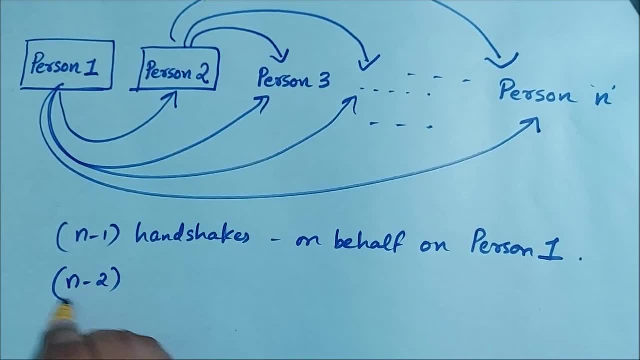 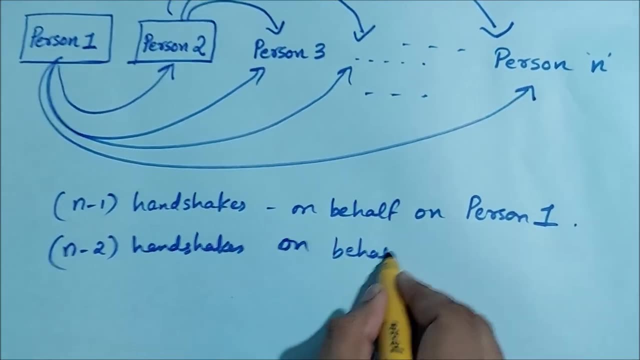 So person 2, on behalf of person 2's handshakes, we will count n minus 1.. We now see that n minus 1 is actually 2 handshakes, because the handshake between person 1 and person 2 were already counted on the behalf of person 1's handshakes, right? 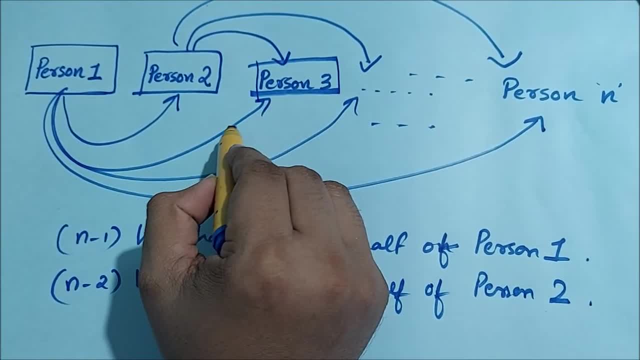 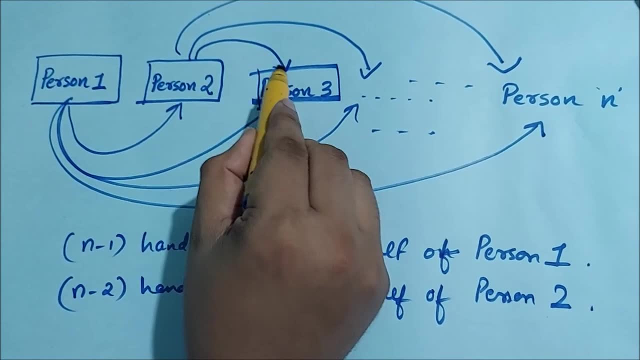 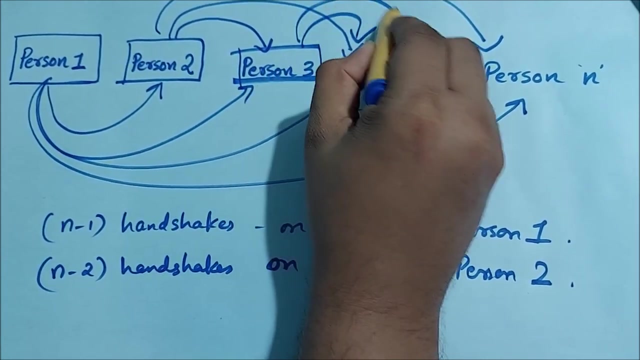 Now, next is the turn for the person 3.. Person 3 will not make handshake with person 2 or person 1, because the handshake between person 2 and person 3 has already happened And the handshake between person 3 and person 1 was also already happened. 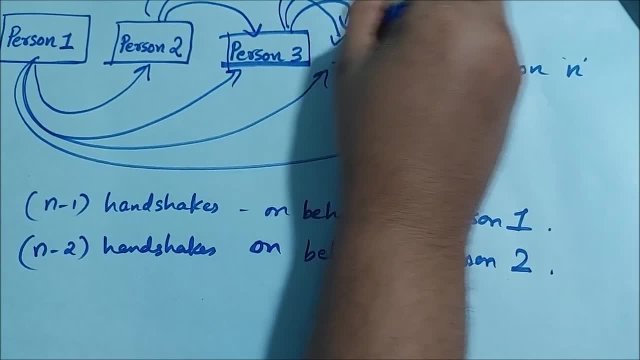 So Person 3 will only make handshake with person 4, person 5 and person 3 will also make handshake with person 3.. and so on till person n. so n minus 3 handshakes will be counted on behalf of person 3's handshakes.